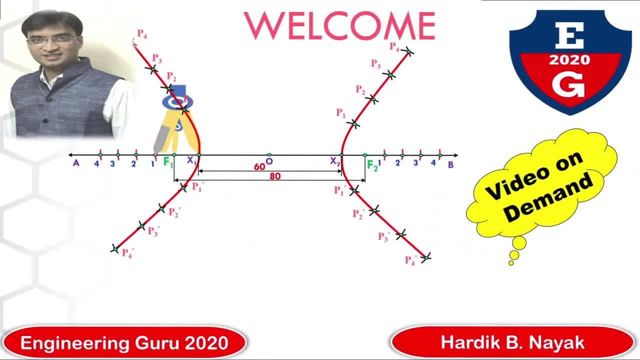 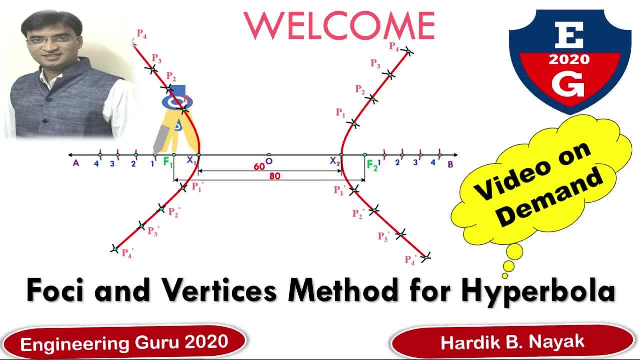 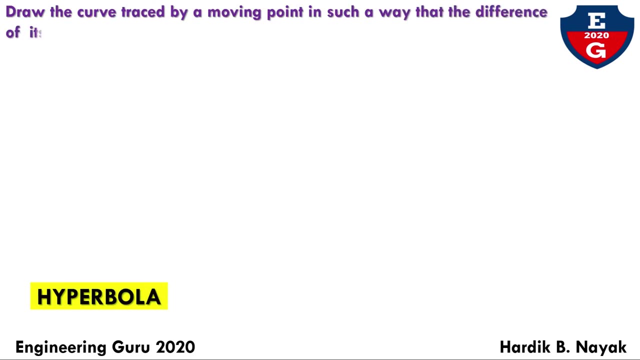 The video will be recorded in a light light setting. The camera will turn on when the light is turned on. The light is on. There is a light on. You will see the light on the camera. Get ready. The camera will turn on when the light is turned on. 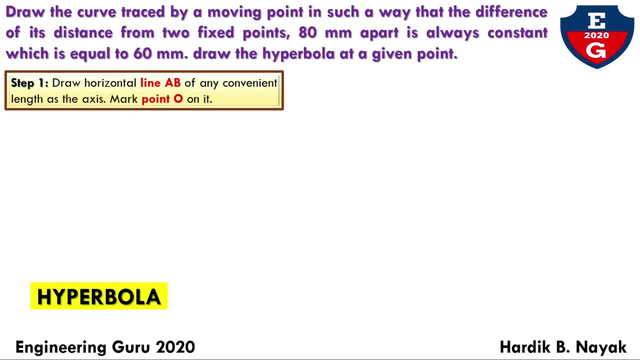 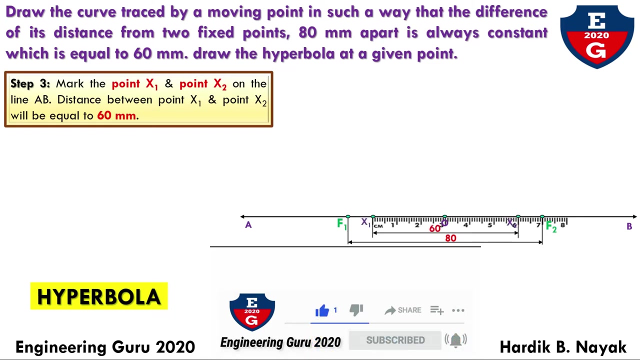 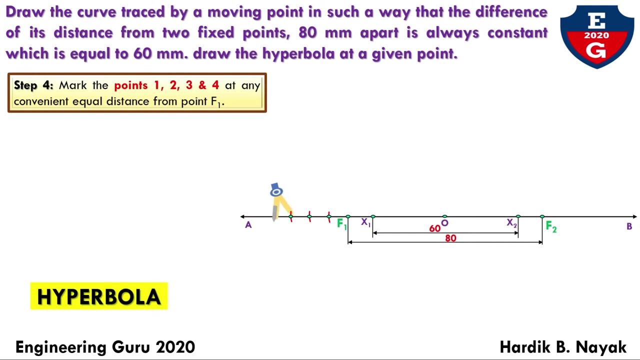